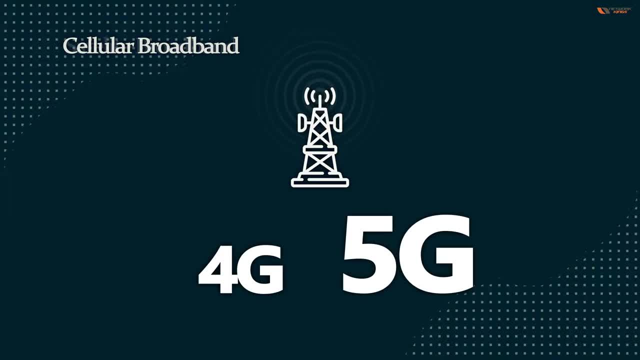 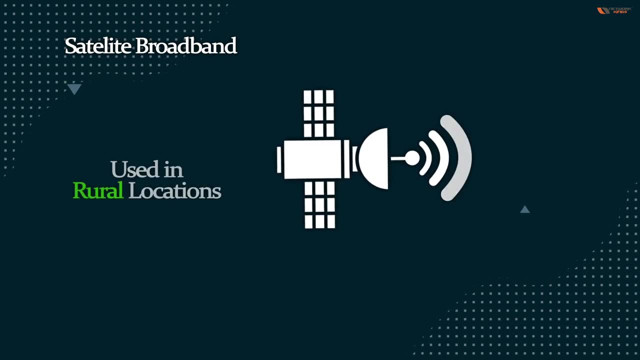 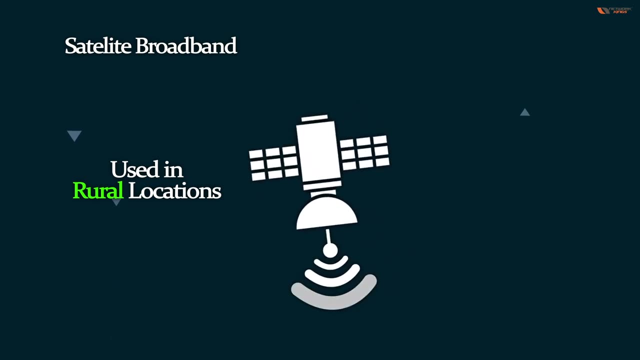 but nowadays the 4g, 5g is more popular. but nowadays we have also satellite broadband also in the market, but it is not for the urban location. mostly it is for rural locations because the speed and all things are not that great. okay, so whenever we talk about wireless, the standard, 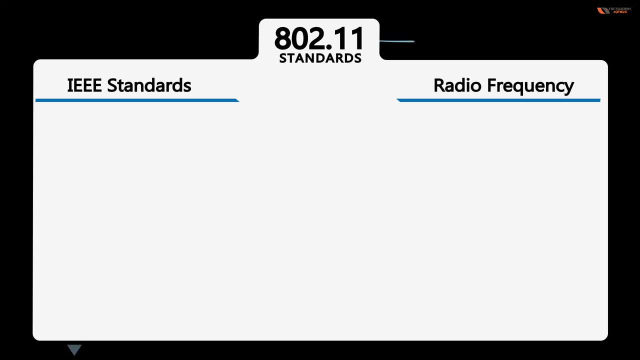 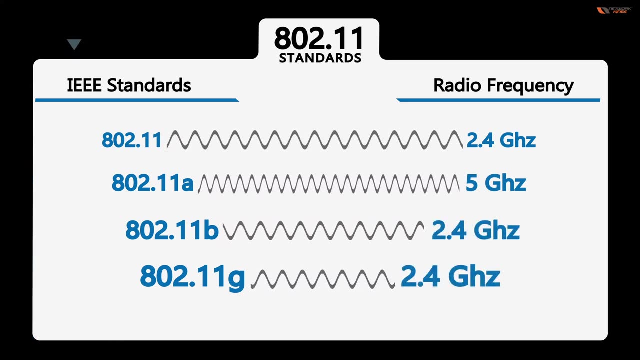 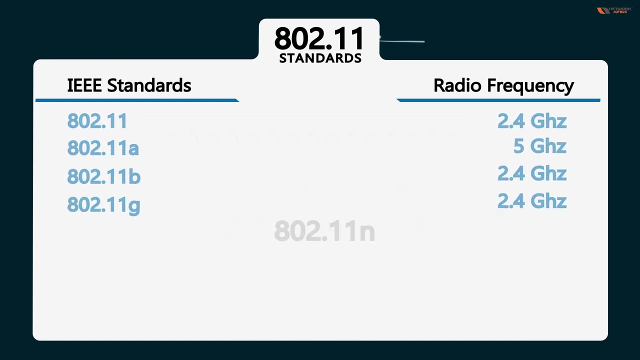 comes 802.11, it means it is a wireless standard. standard means the radio frequency, all the signals of wi-fi radio- okay, we are. all these frequencies are called radio frequencies, okay, and they have standard in wi-fi. the wireless standard is 802.11. till here. they are very old nowadays we are using 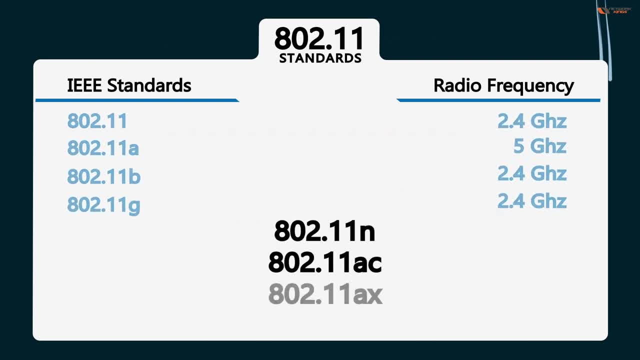 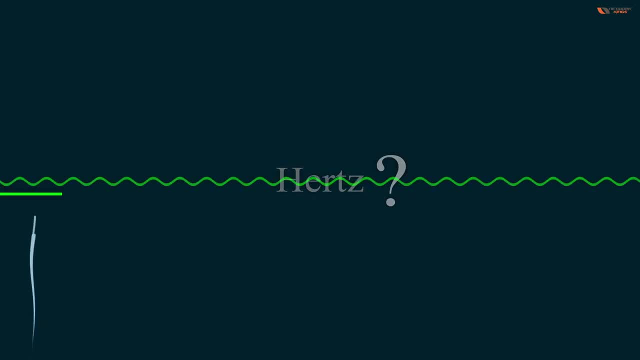 802.11 n, 11 ac, 11 ax- this is the latest- which is called wi-fi 6 also. okay, so, by the way, if you do not know what is hertz, so the number of cycles per second is called wave. so the number of cycles per second is called wave. so the number of cycles per second is called wave. 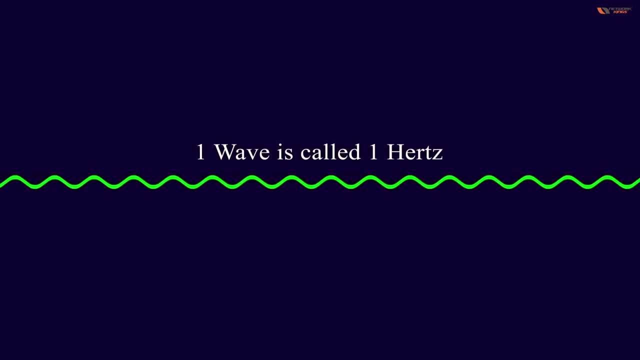 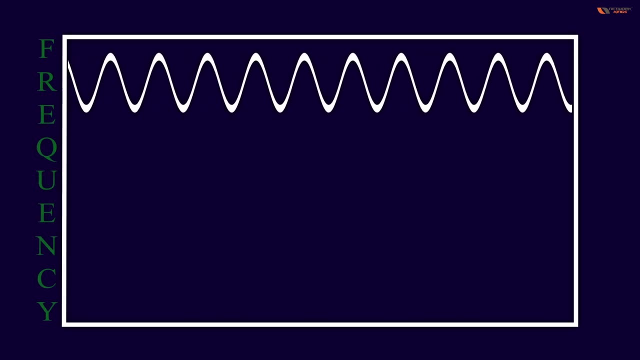 okay, so one wave is called one hertz. this is one wave. okay, this is called one hertz. okay, this is a frequency. but if the frequency is like this, so now you can see per second- you have now more waves. okay, so if we type and we have like this: 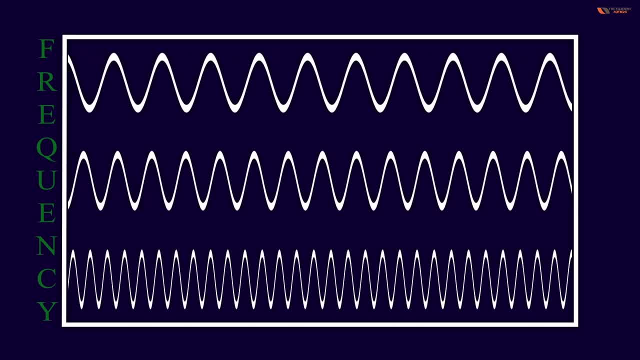 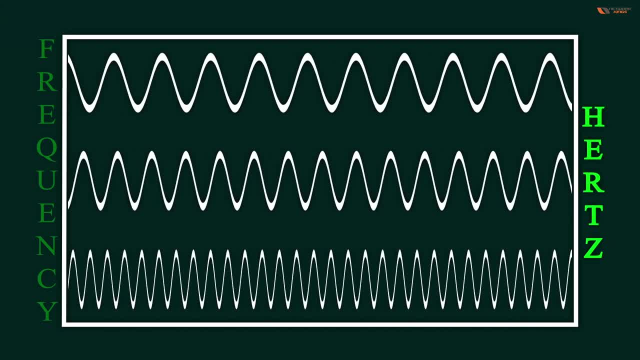 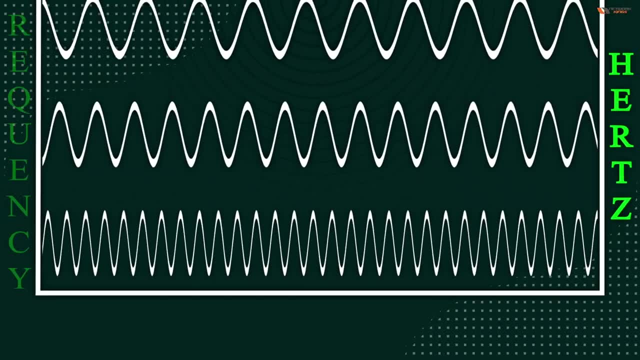 so now you have more waves. okay. so here you have less waves average. now you have higher waves. this is called the hertz. okay, so when you have too much frequency in per second, those are called like megahertz, gigahertz, terahertz, so so if we have one thousand in one second, they are called. one kilohertz. so when you have too much in one second, there are a lot of waves, okay, too much wi-fi signals, they are called megahertz. okay, when you have millions or like billion of waves in one second, is called gigahertz. so your wi-fi is working on 2.4 gigahertz and there is 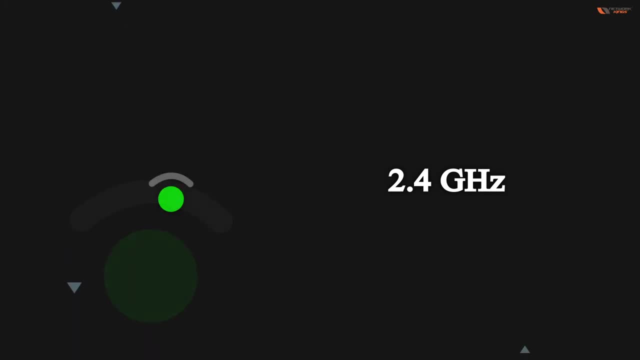 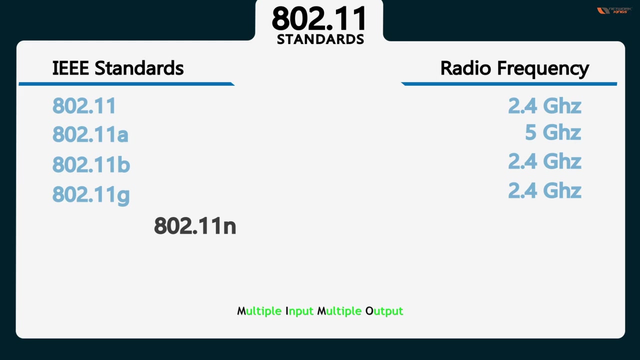 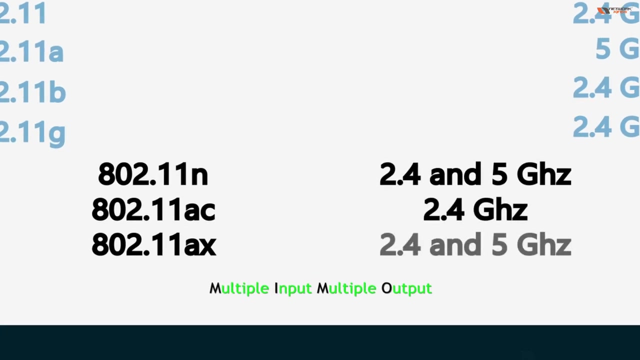 another frequency which is like 5 gigahertz. it means in 2.4 you get this much waves per second second and this if you multiply by 5, it is called 5 gigahertz. so in the latest ranges they have now mimo technology. so this is a 802.11 ac, which is a 5 gigahertz. and this is 802.11 x, which can go: uh 2.4 and 5 gigahertz both and it can go. the speed is going up to in gbps. also in 802.11 ac the speed is very between 450 to 1.3 range, if you have taken.